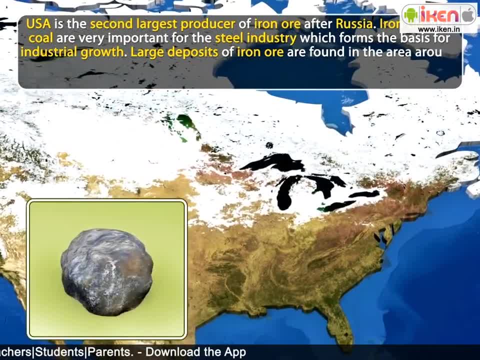 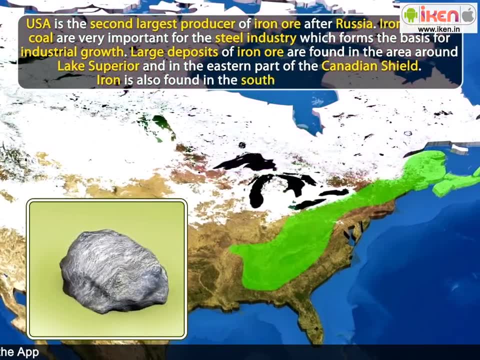 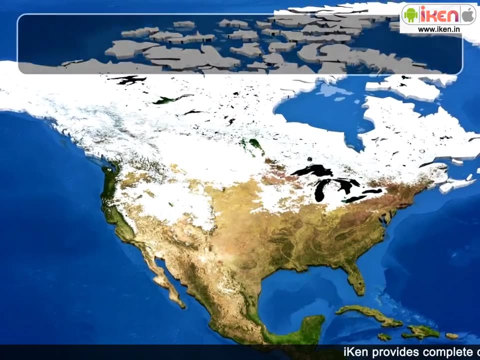 Large deposits of iron ore and coal are also present in the steel industry are found in the area around lake superior and in the eastern part of the canadian shield. iron is also found in the southern appalachians. the united states is the largest producer of copper in the world. it is used in the 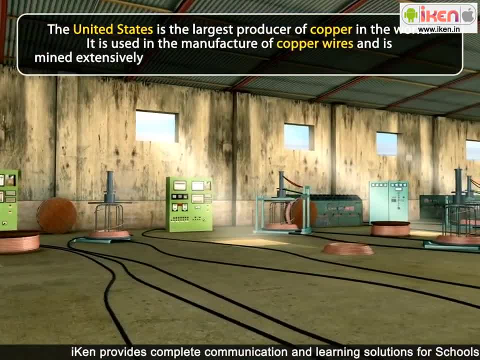 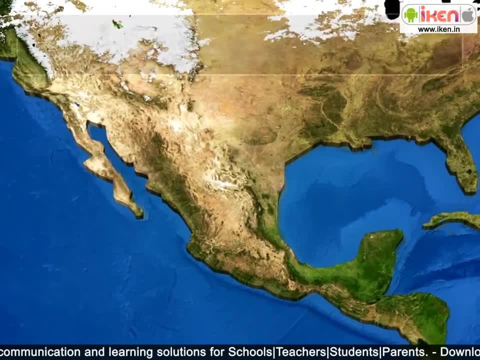 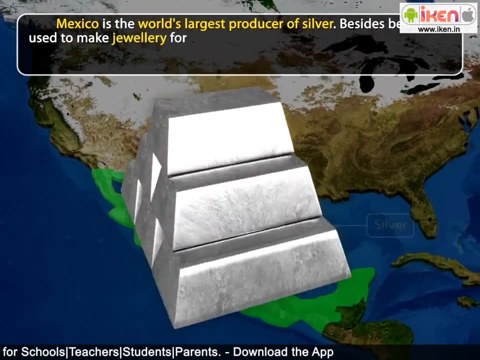 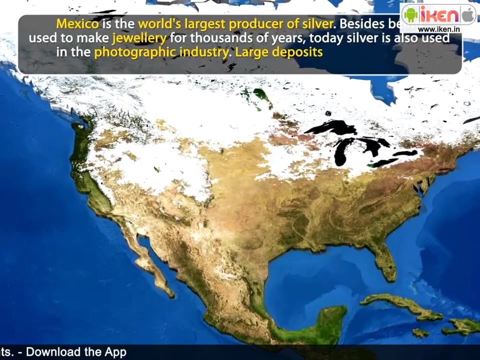 manufacture of copper wires and is mined extensively around the great lakes and the rocky mountains. mexico is the world's largest producer of silver. besides being used to make jewelry for thousands of years, today silver is also used in the photographic industry. large deposits of silver are found in usa and canada. 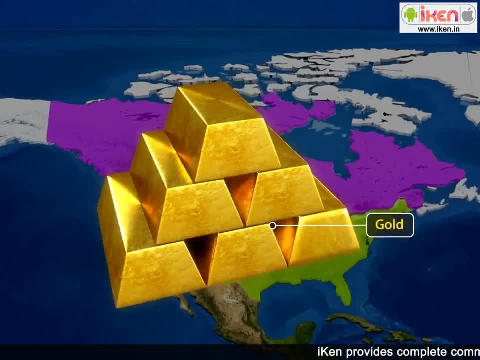 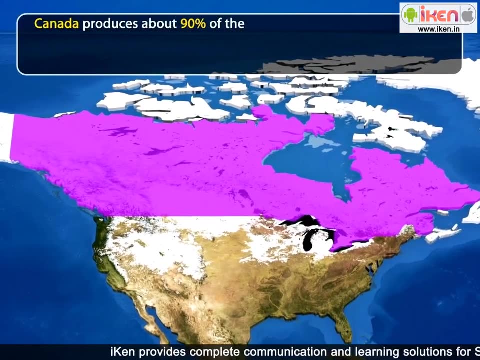 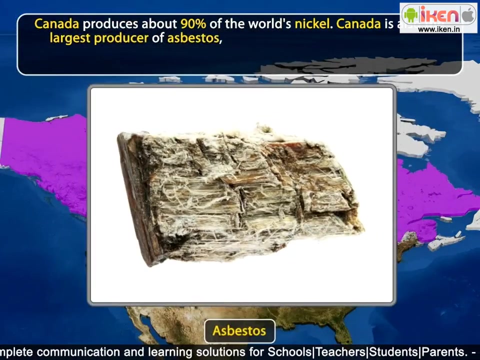 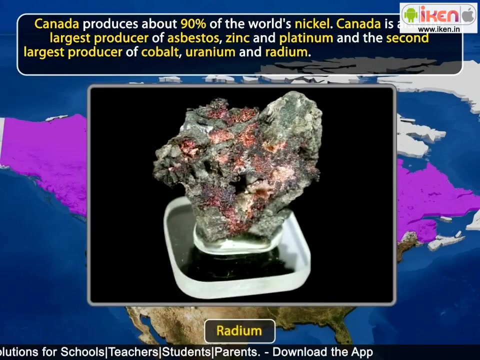 canada and the united states produce substantial amounts of gold, which is mined in the rocky mountains. canada produces about 90 percent of the world's nickel. canada is also the largest producer of asbestos, zinc and platinum and the second largest producer of cobalt, uranium and radium. the united states is the world's largest producer of uranium and sulfur. 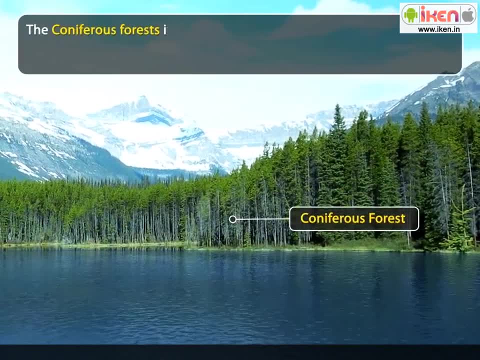 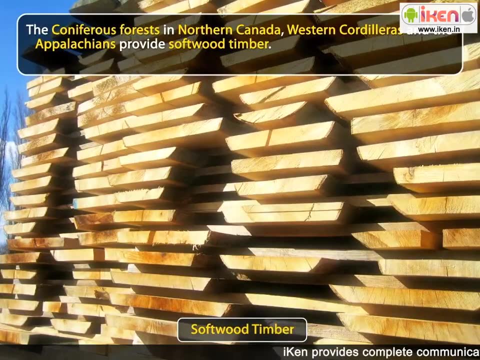 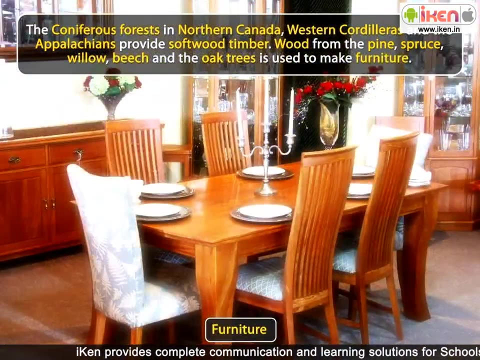 the coniferous forests in northern canada, western cordilleras and the appalachians provide softwood timber. wood from the pine, spruce, willow, beech and the oak trees is used to make furniture. the pine and spruce trees provide wood pulp for the paper industry, as well as raw material for 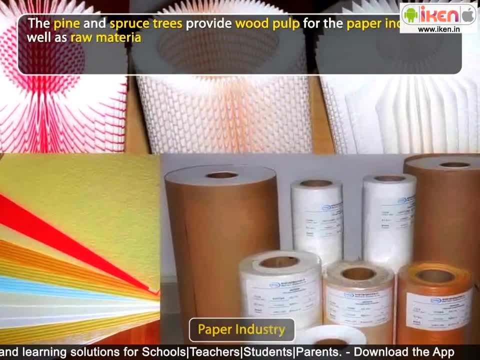 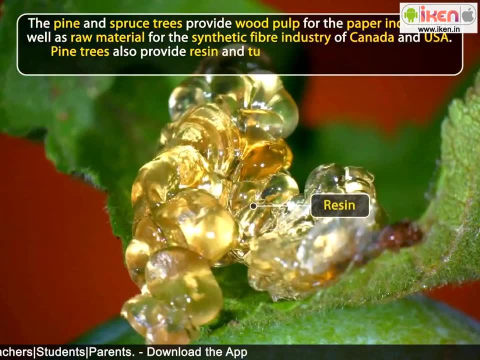 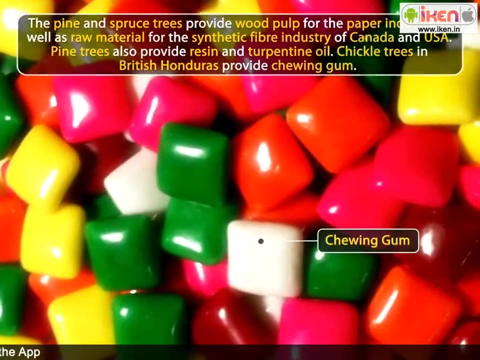 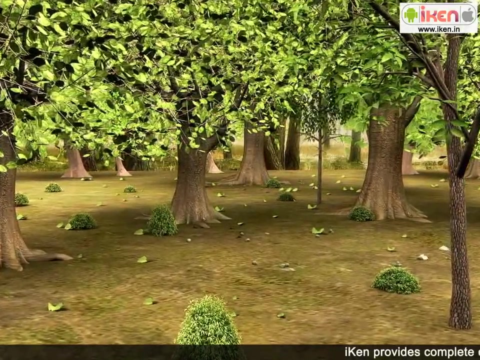 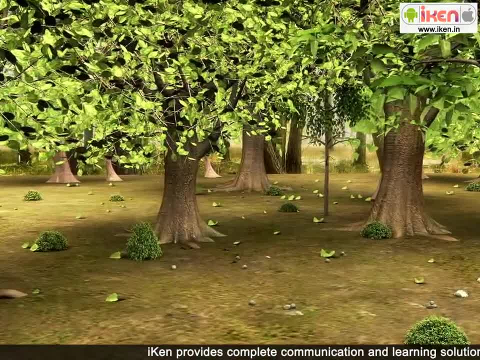 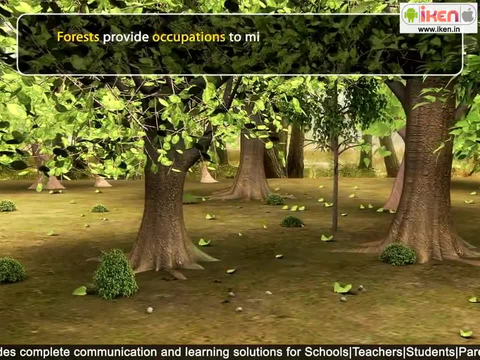 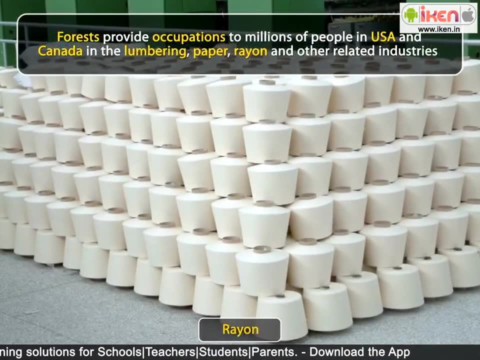 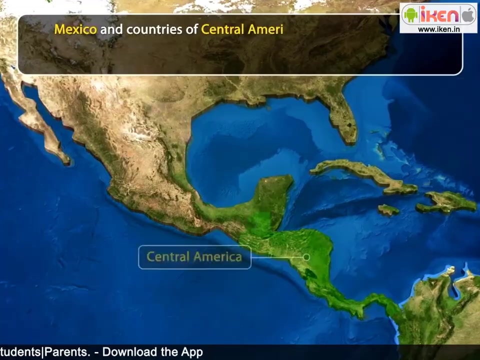 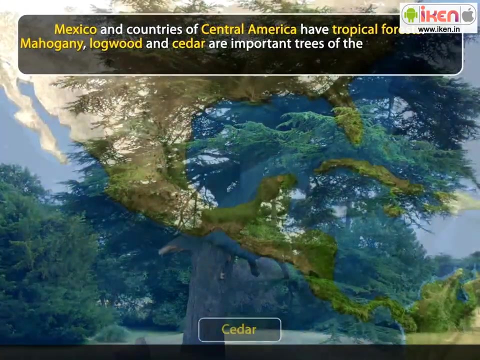 sprint. despite being cut down to provide land for human settlement and cultivation in the past decade, forests provide occupations to millions of people in usa and canada in the lumbering paper, rayon and other related industries. mexico and countries of central america have tropical forests. mahogany, logwood and cedar are important trees of the tropical forests. these are called hardwood trees. 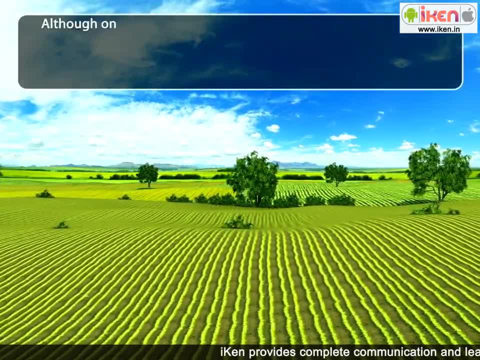 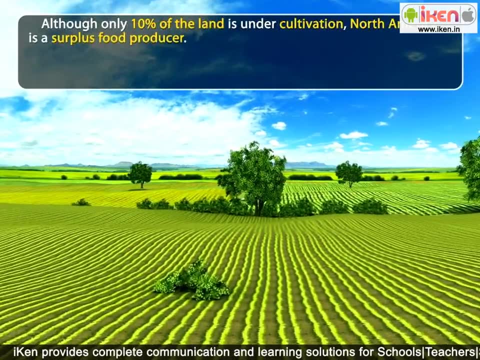 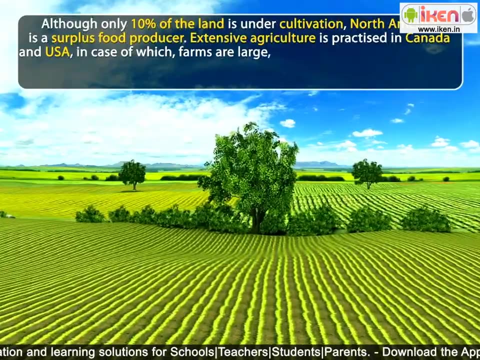 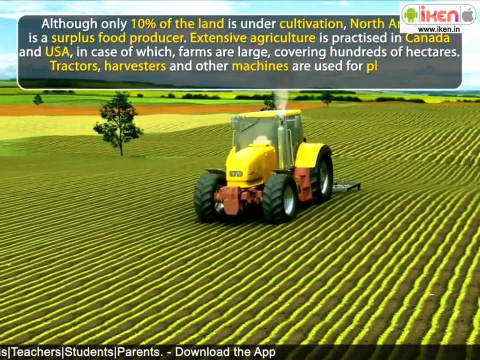 and they are used to make firewood in the natural environment, although only 10 percent of the land is under cultivation. north america is a surplus food producer. extensive agriculture is practiced in canada and usa, in case of which farms are large covering hundreds of hectares. tractors, harvesters and other machines are used for plying and other work on the 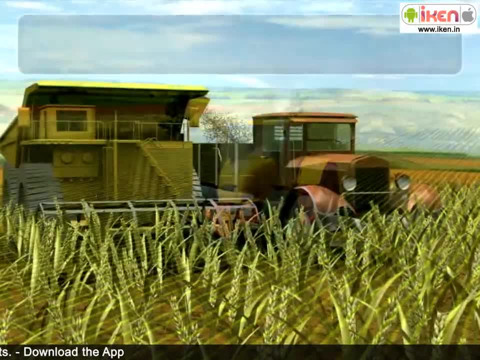 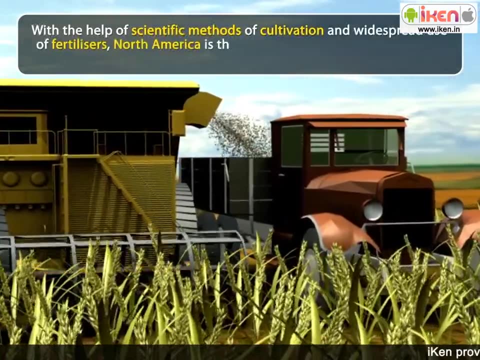 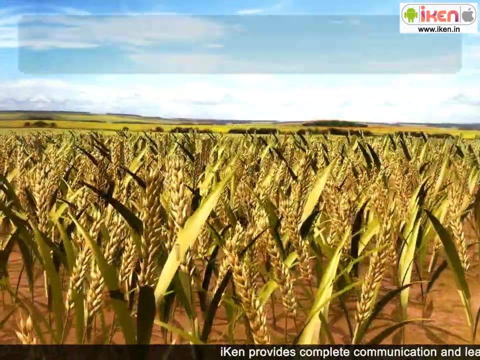 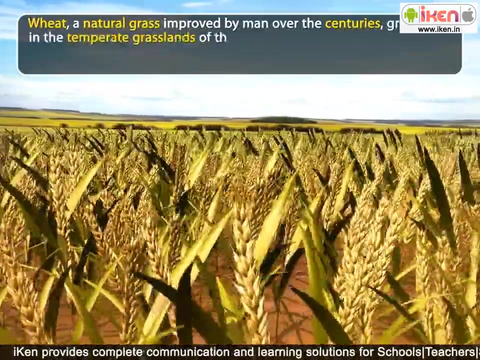 farm with the help of scientific methods of cultivation and widespread use of fertilizers. north america is the world's largest producer of maize wheat and soybeans. wheat, a natural grass improved by man over the centuries, grows well in the temperate grasslands of the world. it is grown extensively in the prairies of north america, where the soil is. 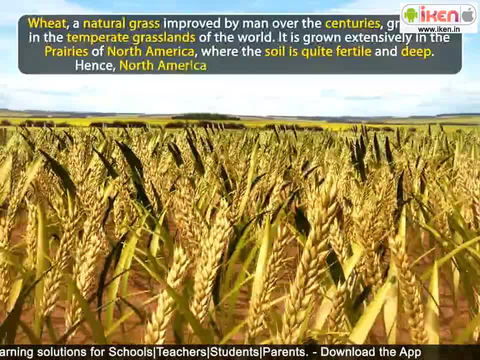 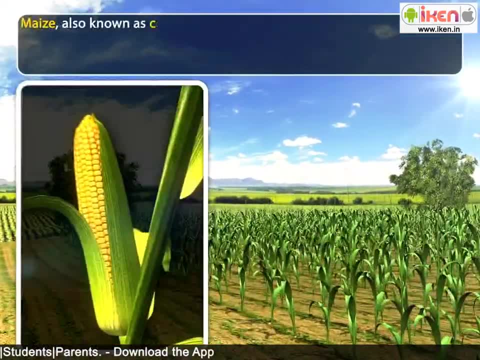 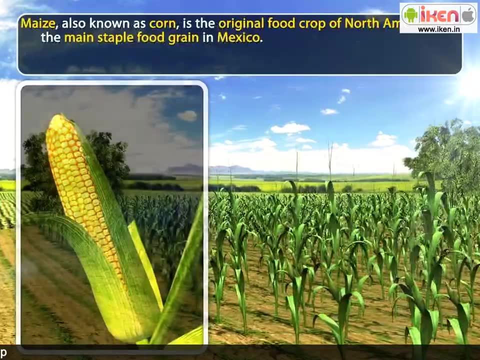 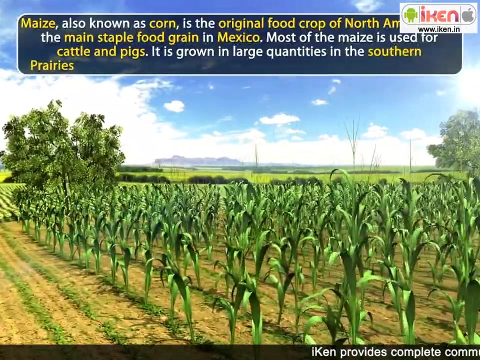 quite fertile and deep. hence north america is the largest producer of wheat. maize, also known as corn, is the original food crop of north america and the main staple food grain in mexico. most of the maize is used for cattle and pigs. it is grown in large quantities in the southern prairies, as it requires a warm climate and frequent showers in summer. 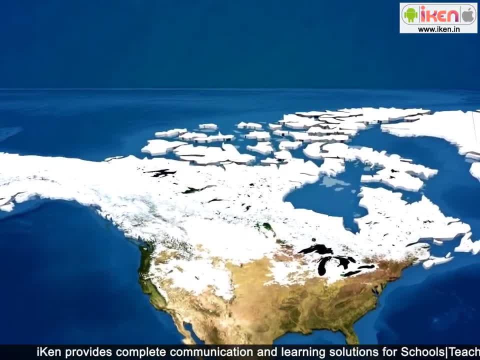 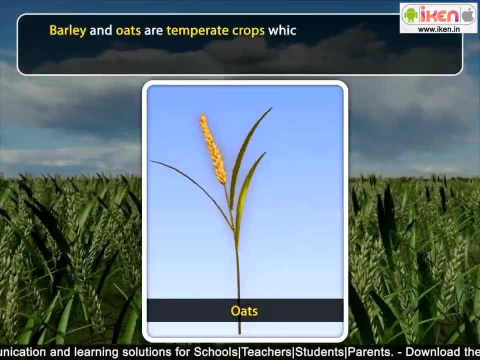 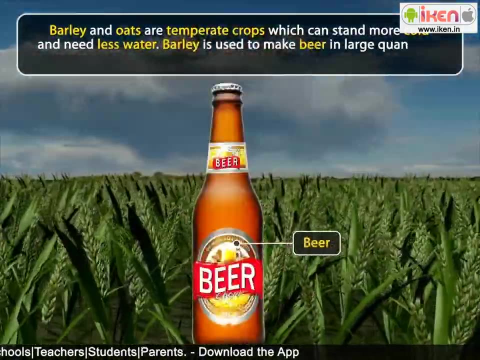 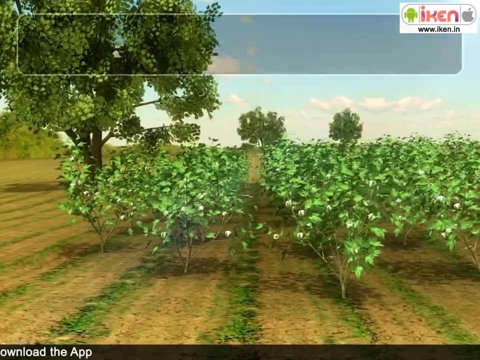 north america produces more than half of the total maize produced in the world. barley and oats are temperate crops which can stand more cold and need less water. barley is used to make beer in large quantities, while oats are used as cattle fodder. cotton grows well in the mississippi basin south of the prairies, as well as 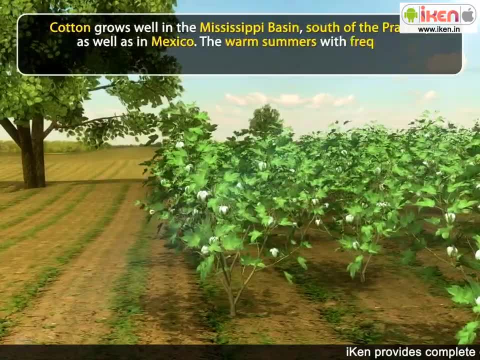 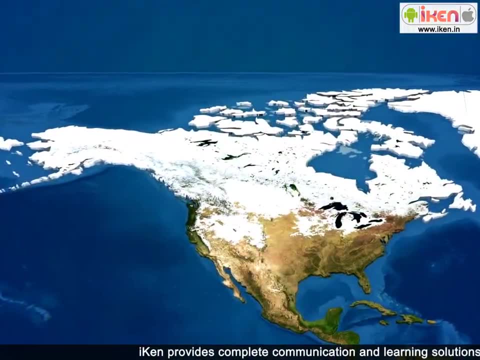 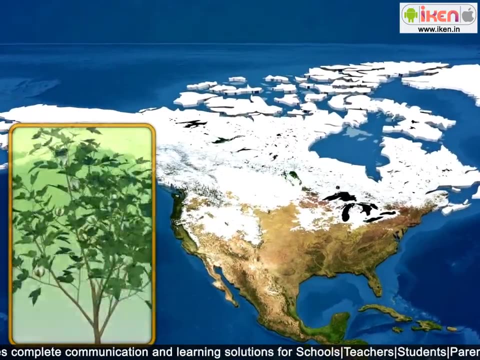 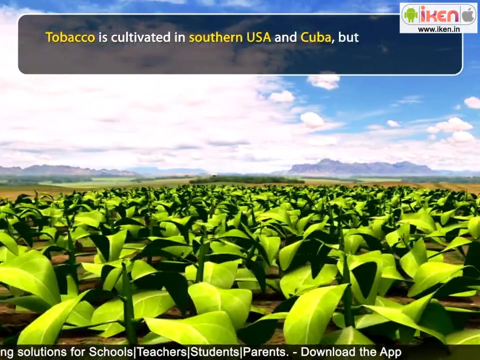 in mexico. the warm summers with frequent rainfall and fertile soil provide suitable conditions for growing cotton. north america is the largest producer of cotton in the world and also produces the superior long staple variety. tobacco is cultivated in southern usa and cuba, but some of the best varieties are grown in north america. 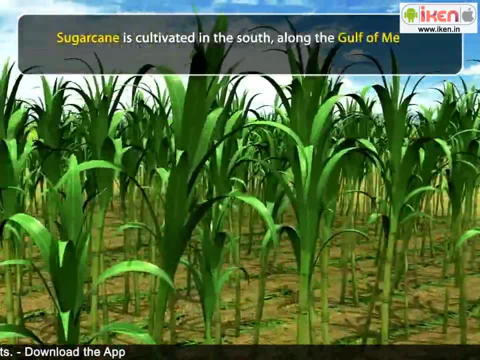 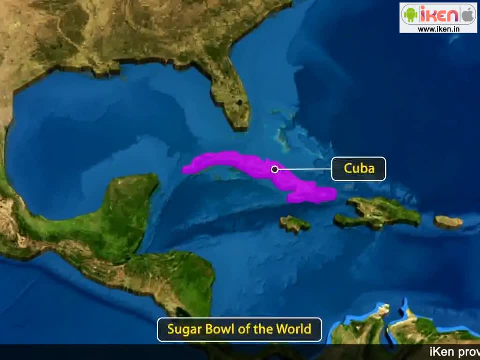 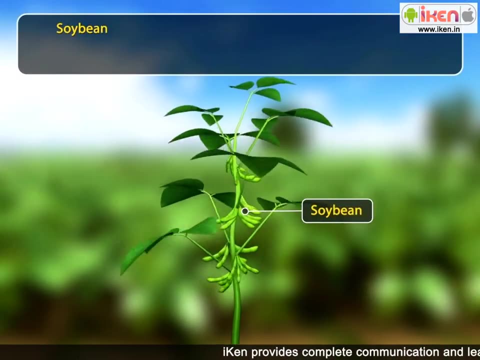 sugarcane is cultivated in the south, along the gulf of mexico, parts of central america and the west indies. cuba, known as the sugar bowl of the world, is the world's largest exporter of sugar. soybean is an important crop that is grown in the same areas as maize. 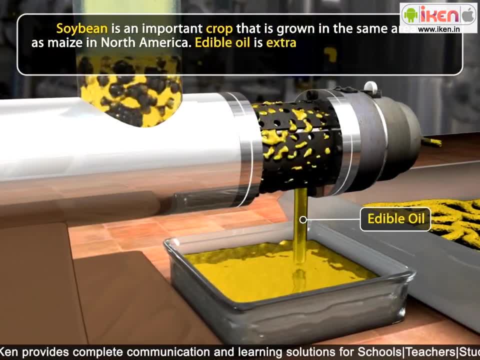 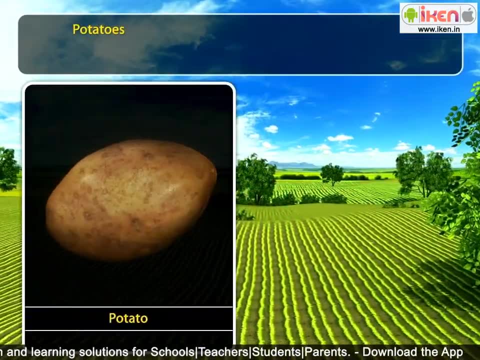 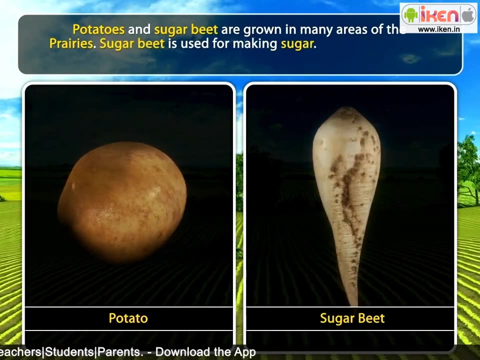 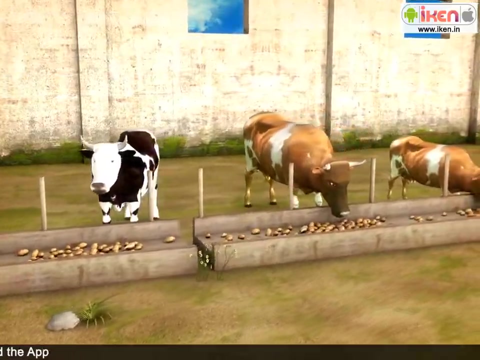 in north america. edible oil is extracted from the beans with the help of heavy machines. potatoes and sugar beet are grown in many areas of the prairies. sugar beet is used for making sugar. both the crops are used to feed cattle and pigs, just like sugarcane rice is also cultivated in the southern parts of north. 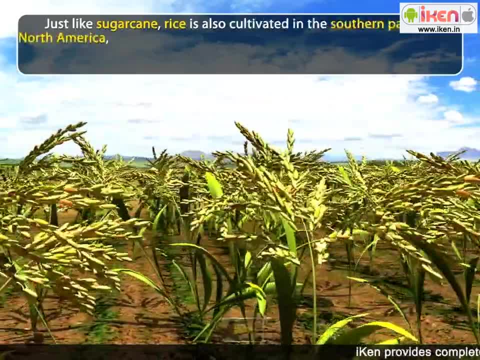 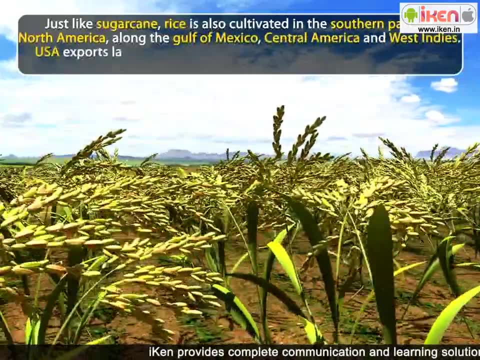 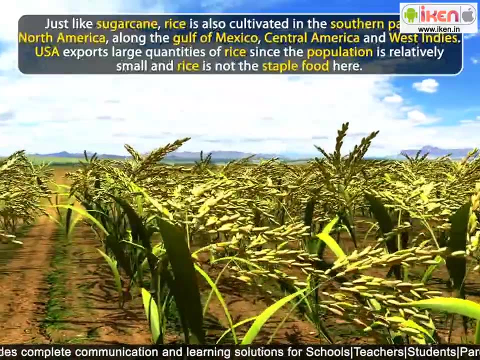 america along the gulf of mexico, central america and west indies. usc has grown in many areas and is also commonly used in the south of america, exports large quantities of rice, since the population is relatively small and rice is not the staple food here. fruits are cultivated in California around the 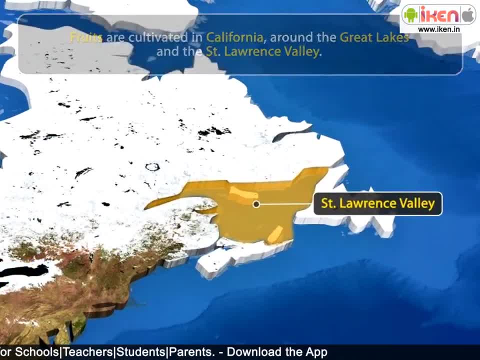 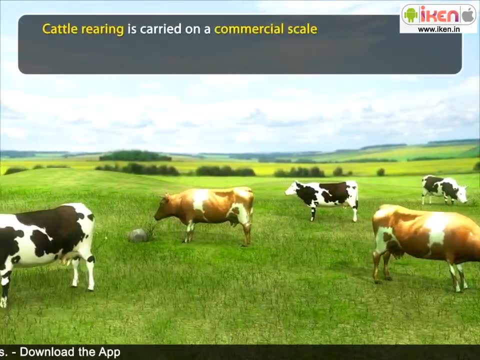 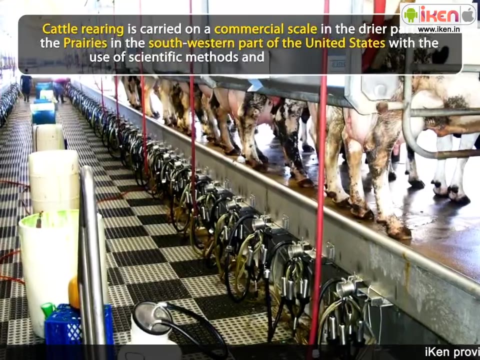 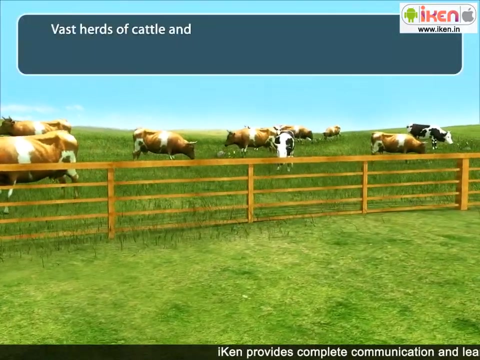 Great Lakes and the st Lawrence Valley. cattle rearing is carried on a commercial scale in the drier parts of the prairies in the southwestern parts of the United States with the use of scientific methods and modern technology. vast herds of cattle and sheep are kept on large ranches. cattle rearing has now 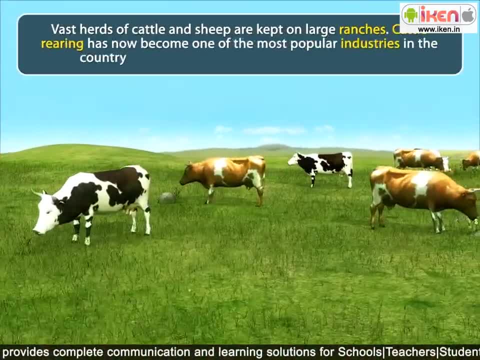 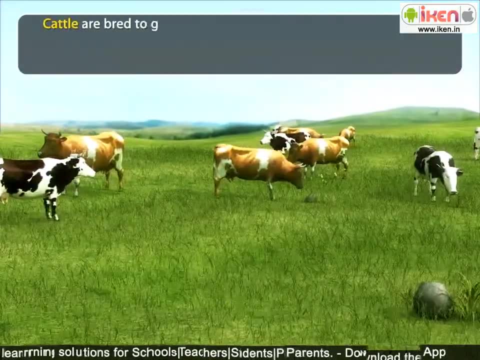 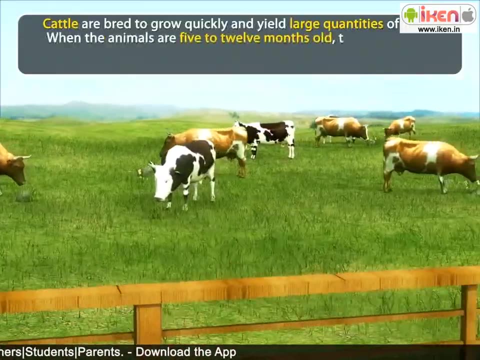 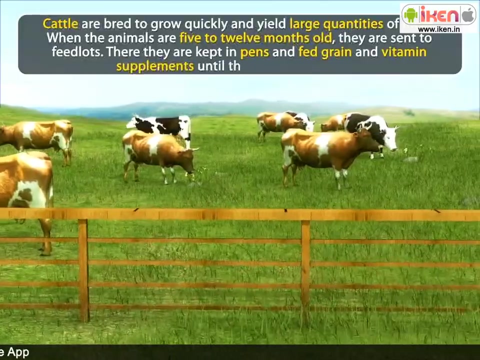 become one of the most popular industries in the country, considering its usefulness as well as revenue. cattle are bred to grow quickly and yield large quantities of rice in the United States. when the animals are five to twelve months old, they are sent to feedlots. there they are kept in pens and fed grain and vitamin supplements until they 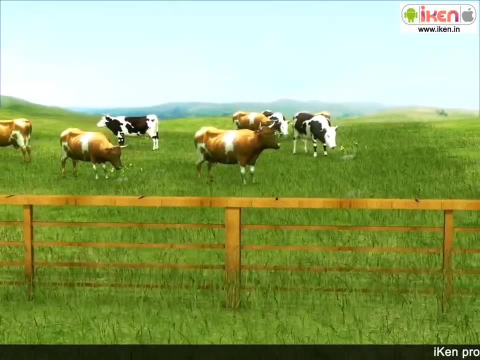 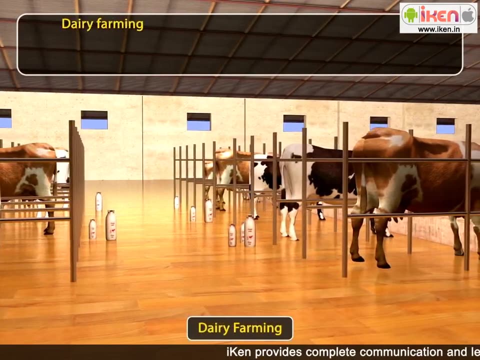 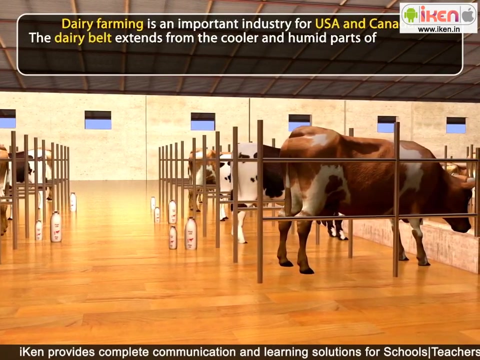 reach market size. North America is the largest producer of meat, with about one-fourth of the world's production. dairy farming is an important industry for USA and Canada. the dairy belt extends from the cooler and humid parts of the prairies through the Great Lakes area to the northeast region along the 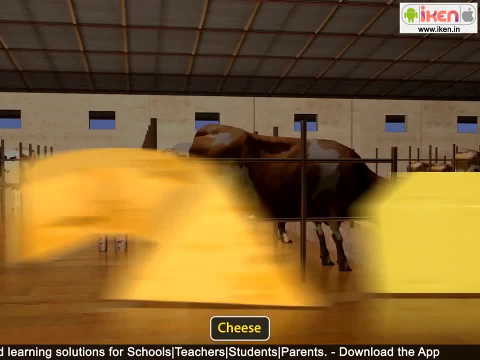 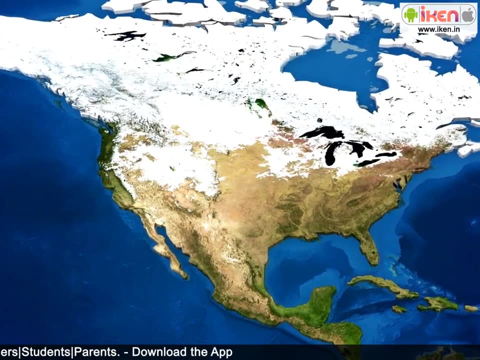 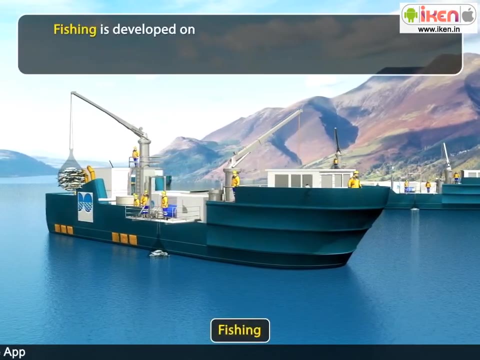 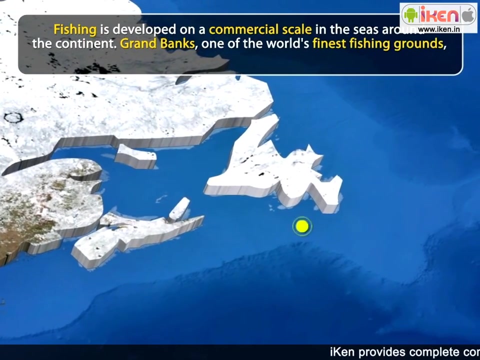 Atlantic coast. milk, cheese and butter are the chief products. North America produces about 25% of the world's total milk and dairy products. fishing is developed on a commercial scale in the seas around the continent. Grand Banks, one of the world's finest fishing grounds, is known for its high-quality dairy products. 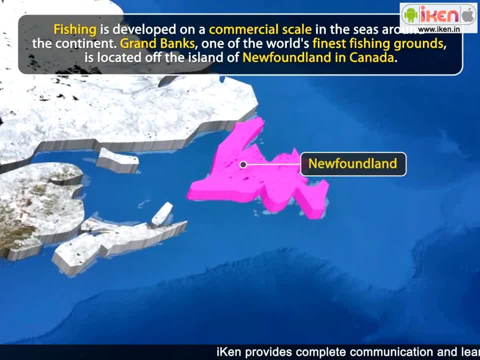 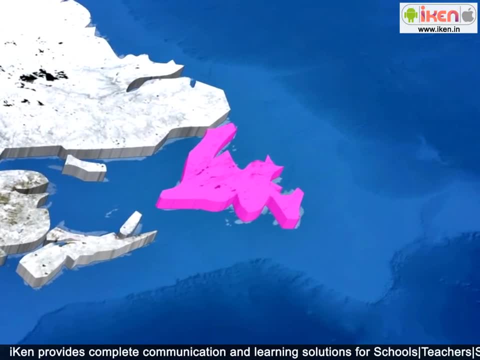 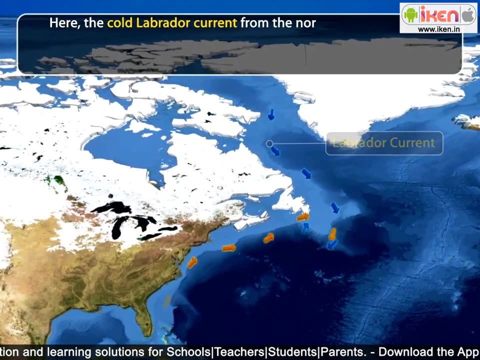 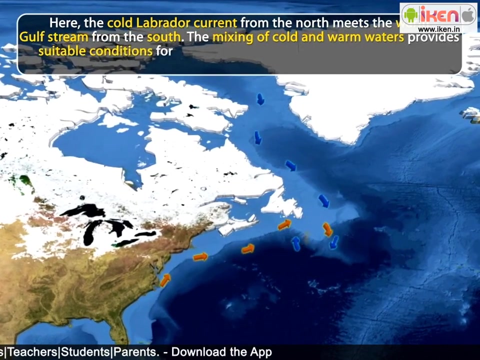 located off the island of Newfoundland in Canada. it has an extensive continental shelf, making the water shallow enough for the sunlight to reach the bottom. here the cold labrador current from the north meets the warm Gulf Stream from the south. the mixing of cold and warm waters provides suitable conditions for fish to 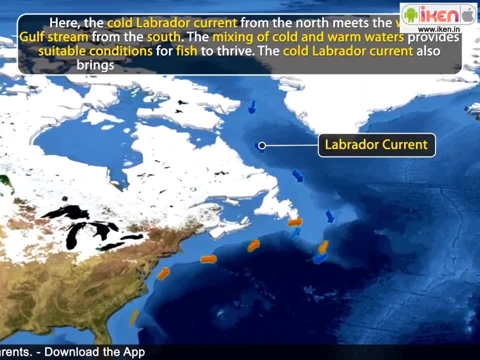 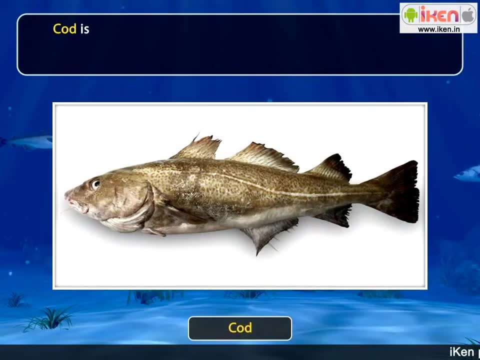 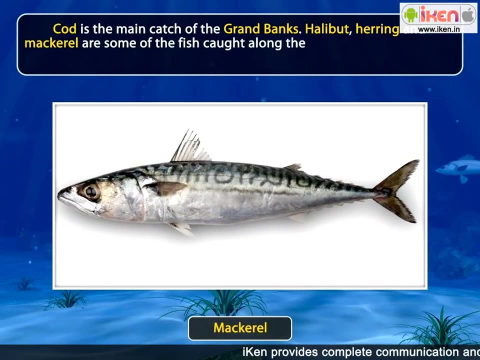 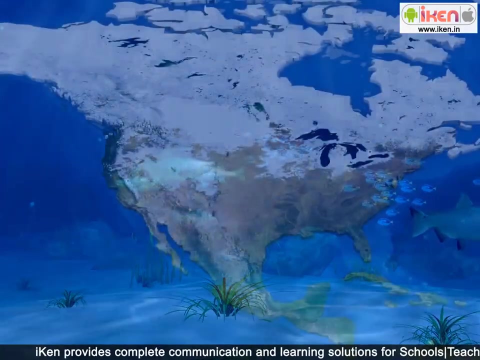 thrive. the cold labrador current also brings plenty of plankton and which provides food for fish. cod is the main catch of the Grand Banks. halibut, herring and mackerel are some of the fish caught along the Atlantic coast. salmon is the main fish of the Pacific Coast. North America is rich in water. 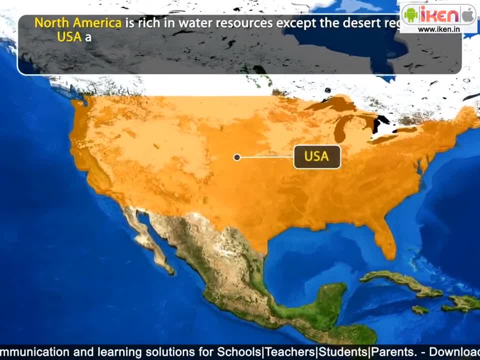 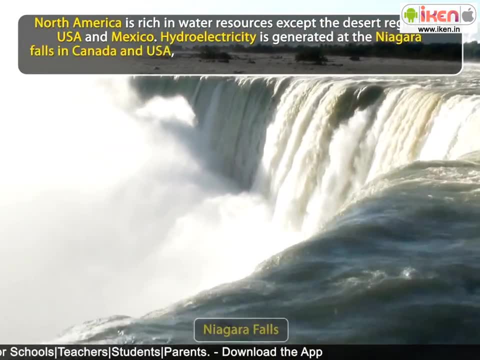 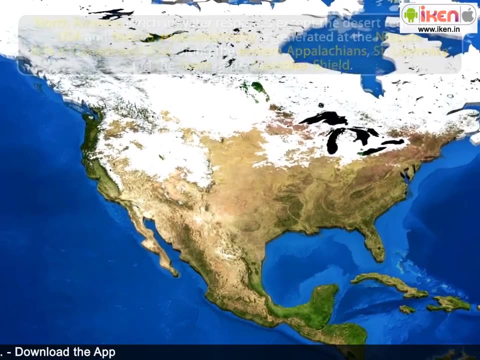 resources. except the desert regions of USA and Mexico, hydroelectricity is generated by the use of hydroelectric power plants at the Niagara Falls in Canada and USA, along the Eastern Appalachians, st Lawrence and the rivers of the Canadian Shield. North America is now the largest.